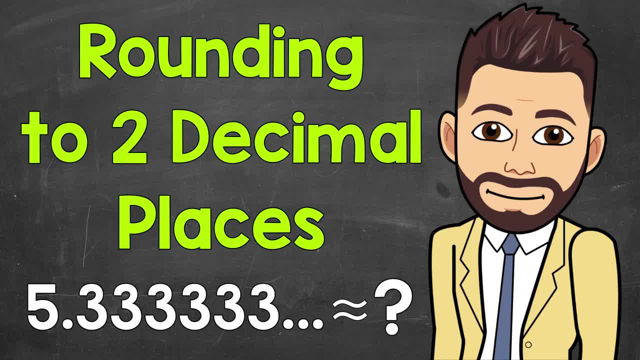 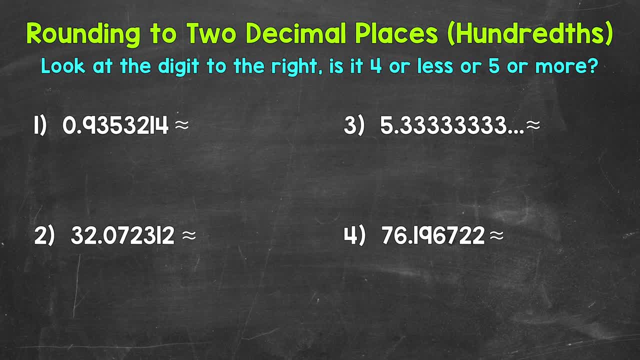 Welcome to Math with Mr J. In this video I'm going to cover how to round to two decimal places, which is rounding to the hundredths place. Now rounding shows up all throughout math and really life as well. So being able to round is important, no matter what class, level of math or goal you are working. 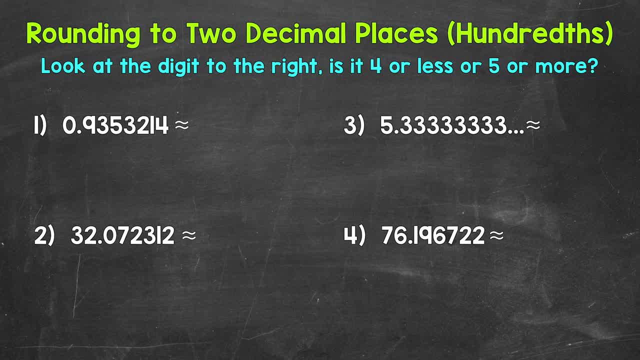 towards Rounding helps us make numbers simpler and easier to work with. Let's jump into number one, where we have a fairly long decimal, We need to round to two decimal places. In other words, we are going to cut this decimal off after two decimal places. the hundredths place We do this. 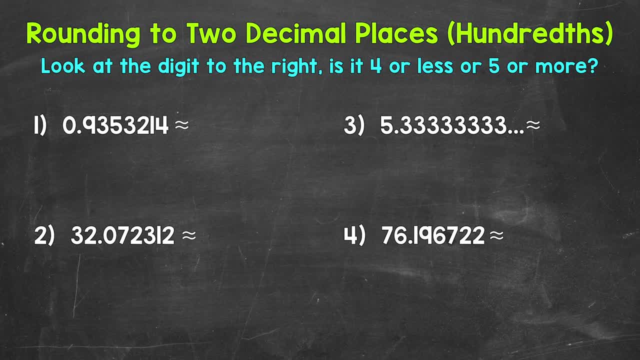 by taking a look at the digit in the hundredths place or whatever other place we want to round to, and then take a look at the digit to the right. That digit to the right tells us if we keep the digit the same or if we round up Four or less. 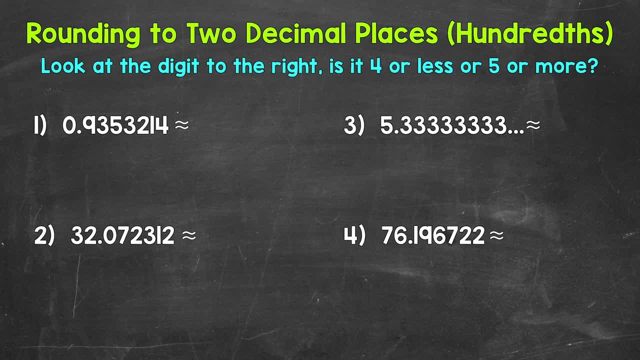 Keep the digit the same: Five or more Round up. I'm going to start by underlining the digit in the hundredths place, which is two spots to the right of the decimal. We have a three in the hundredths place. Take a look to the right, in the thousandths place, We have a five. Basically, 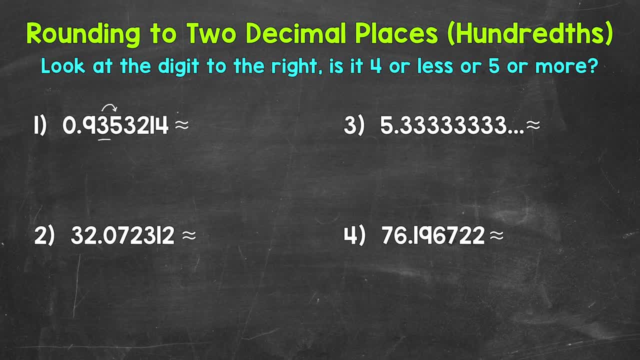 we are seeing if this is closer to ninety-three hundredths or ninety-four hundredths. That digit to the right tells us this: We have a five. Five is five or more, so we round up, This decimal rounds to ninety-four hundredths. 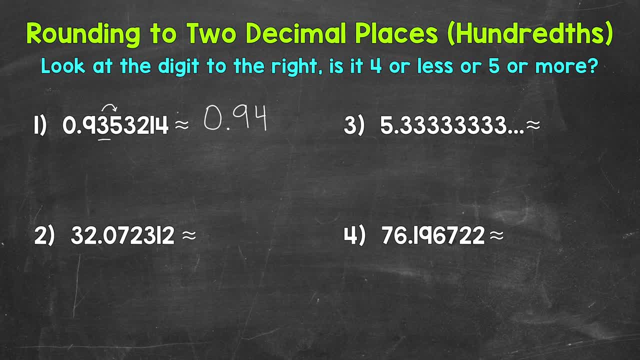 So our original decimal is approximately, or rounds to ninety-four hundredths. We can think of this as cutting the decimal off after two decimal places, so after the hundredths place, And we do this by rounding. Now, this is the approximate sign. We use this. 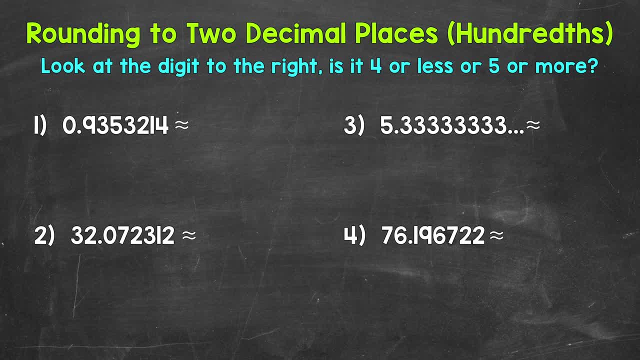 being able to round is important, no matter what class level of math or goal you are working towards. Rounding helps us make numbers simpler and easier to work with. Let's jump into number one, where we have a fairly long decimal, We need to round to two decimal places, In other words. 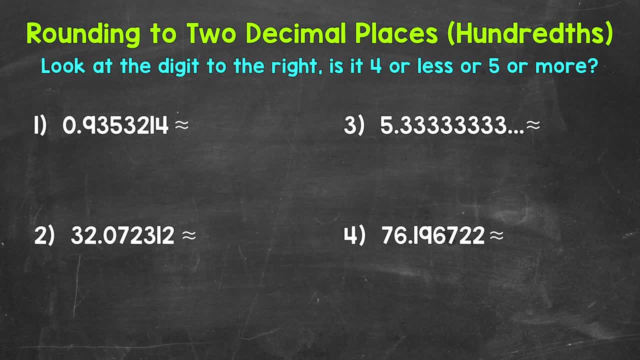 we are going to cut this decimal off after two decimal places, the hundredths place. We do this by taking a look at the digit in the hundredths place or whatever other place we want to round to, and then take a look at the digit to the right. That digit to the right tells us if we 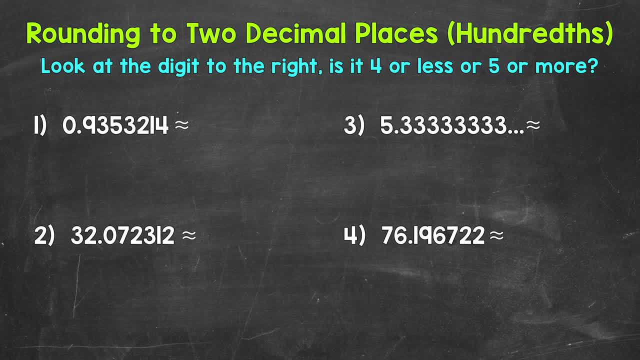 keep the digit the same. or if we round up Four or less, Keep the digit the same: Five or more Round up. I'm going to start by underlining the digit in the hundredths place, which is two spots to the right of the decimal. We have a three in the 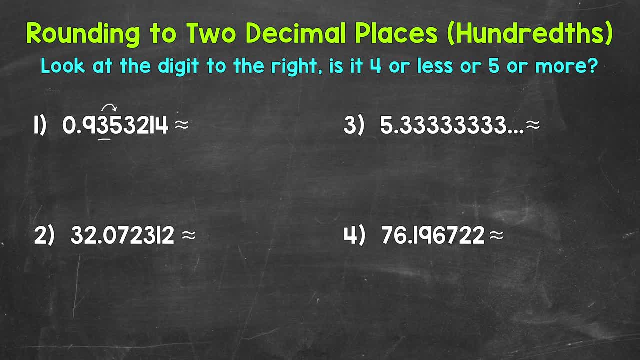 hundredths place. Take a look to the right. in the thousandths place We have a five. Basically, we are seeing if this is closer to ninety-three hundredths or ninety-four hundredths. That digit to the right tells us this: We have a five. 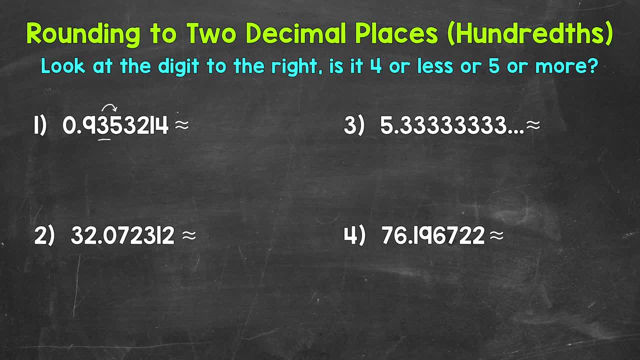 Five is five or more. so we round up This decimal rounds to ninety-four hundredths. So our original decimal is approximately, or rounds to ninety-four hundredths. We can think of this as cutting the decimal off after two decimal places, so after the hundredths place. 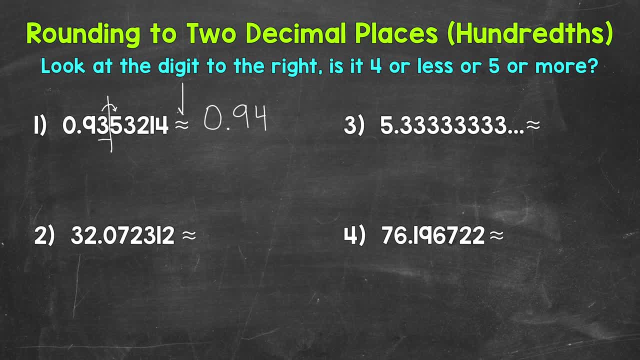 And we do this by rounding. Now, this is the approximate sign. We use this because ninety-four hundredths is a rounded decimal. It's not exactly equal to our original decimal, So we use that approximate sign to show that we have an approximate rounded decimal. 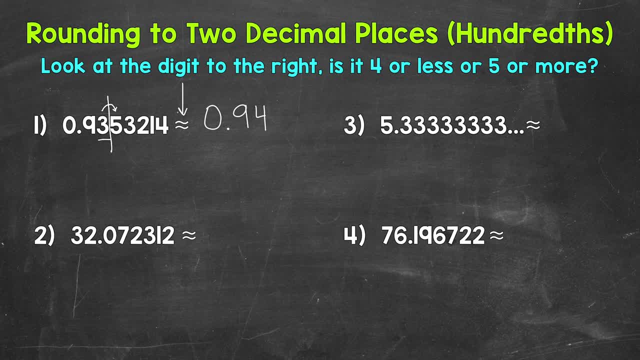 Let's move on to number two, where we have thirty-two and then some decimal digits. There's a seven in the hundredths with a two to the right in the thousandths. Two is four or less, so we stay the same. This decimal rounds to. 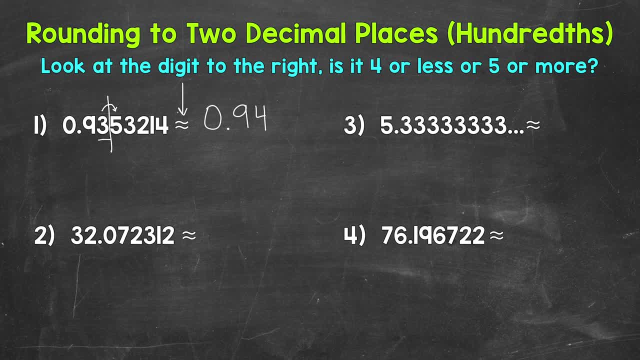 because ninety-four hundredths is a rounded decimal. It's not exactly equal to our original decimal, So we use that approximate sign to show that we have an approximate rounded decimal. Let's move on to number two, where we have thirty-two and then some decimal digits. There's